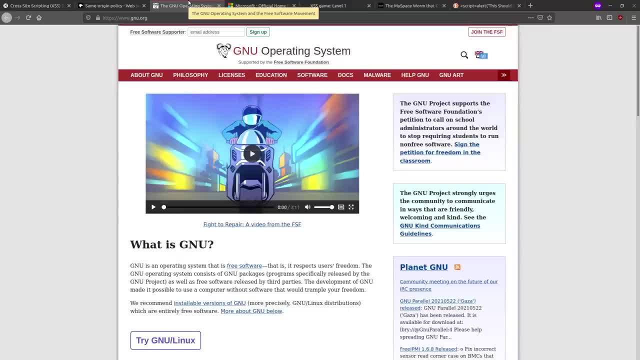 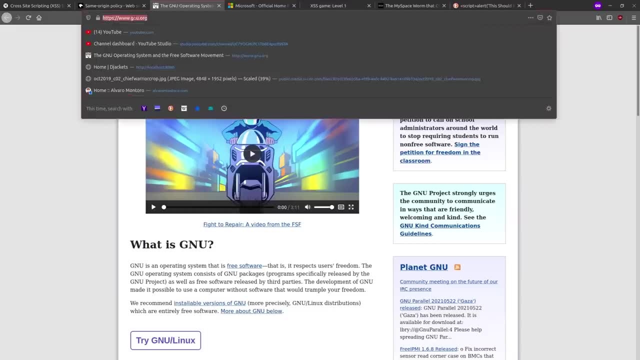 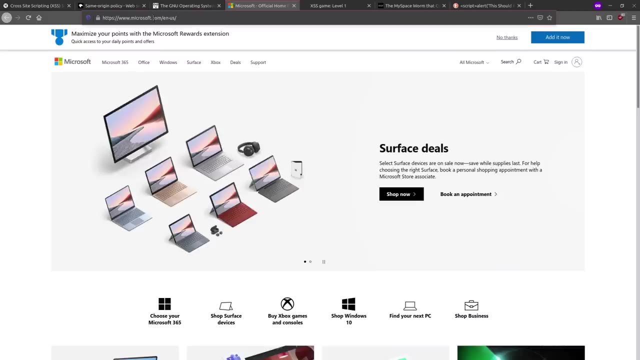 GNUorg, it wouldn't allow reads or writes from Microsoftcom, even though they're both using the same protocol. they're both using HTTPS, but the origin is different, right? This is coming from GNUorg and this is coming from Microsoftcom. Now let's say that you are somehow able to control. 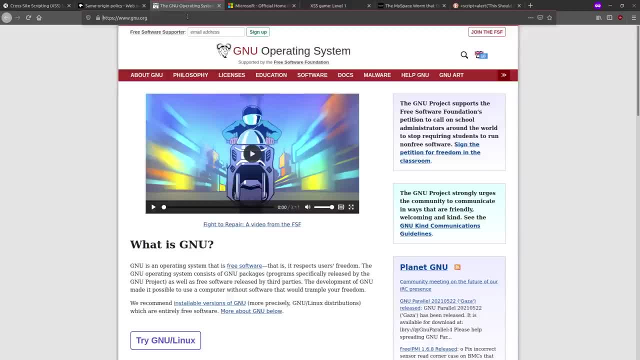 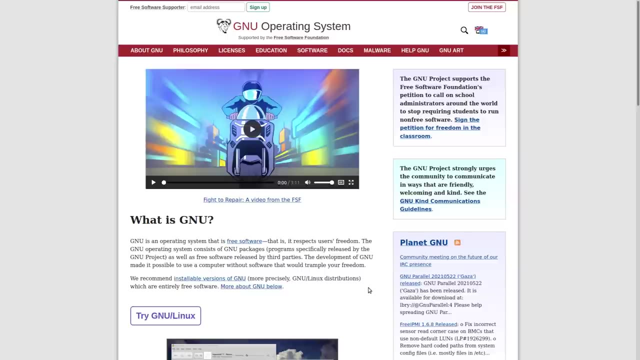 the JavaScript on GNUorg. The JavaScript is able to manipulate the HTML via the DOM APIs and, of course, HTML is the framework for websites. so all of the text, links, pictures and formatting that's done in HTML. In the background is CSS, which JavaScript can manipulate. 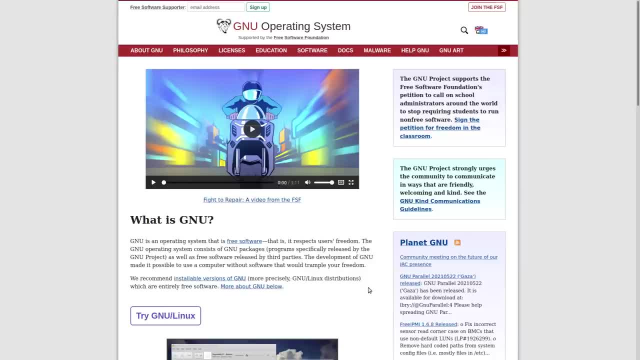 as well. So with control of the JavaScript, you could do something as harmless as just messing up the world. So let's say that you are able to control the JavaScript. on GNUorg, The JavaScript is able to manipulate the HTML via the DOM APIs and, of course, HTML is the framework for websites. 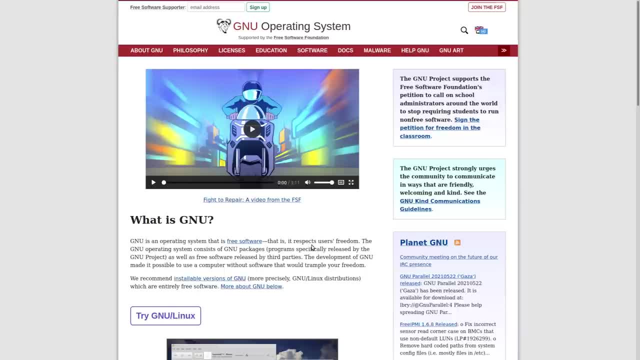 so all of the text, links, pictures and formatting that's done in HTMLorg, The web page you know, fill it with some silly memes, or I guess maybe if you wanted to really troll GNU you would fill it with like Microsoft and different proprietary things. 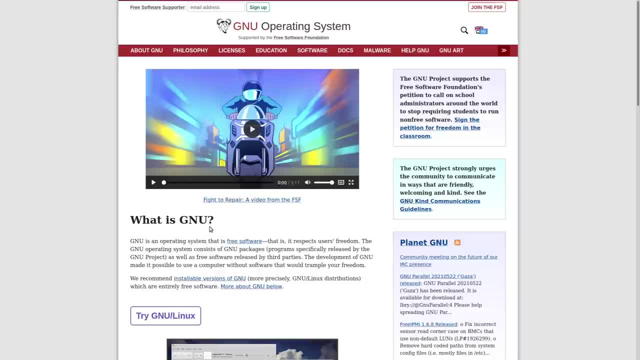 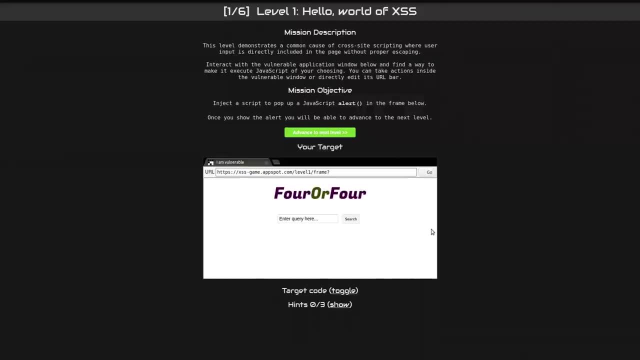 Or you could inject your own JavaScript into the page and have it execute. So over here we have an example of something that is vulnerable to cross-site scripting. So this is just like a simple little search bar, like you would see on all different sorts of websites. 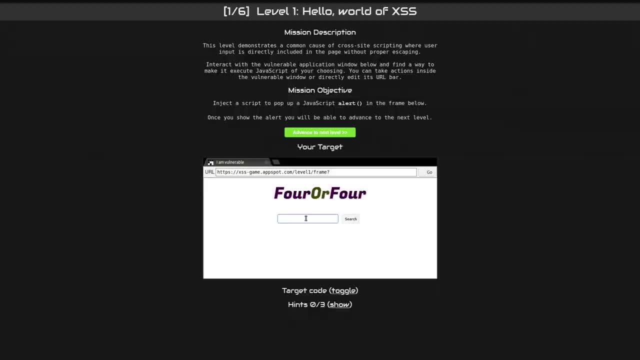 What it's going to do whenever you put something into it is it's going to send an HTTP request containing whatever you put in here. So, like you know, you search for hats. This isn't really connected to anything, but you know what I mean If you were on amazoncom and you search for hats. 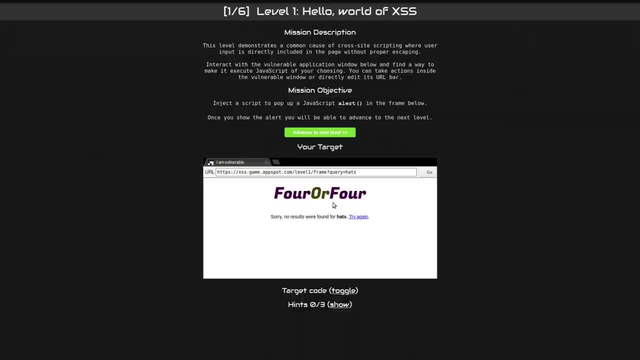 then it would serve you up a different HTML page that's relevant to your search query, So it would show you a bunch of hats that are for sale. But what if I were to send some code and instead of just a normal search query? so, for example, I'm going to do this: 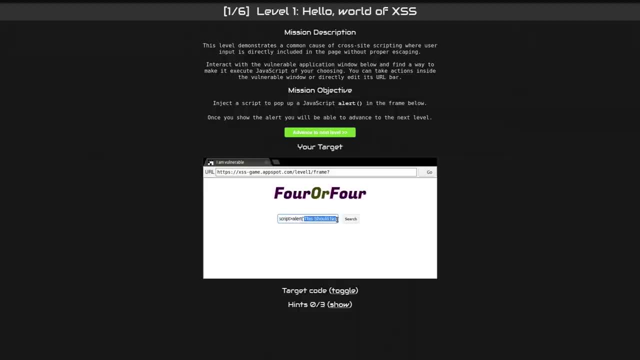 which is going to make an alert pop up and show this should not happen, written inside the alert. And so there you go, And it has some extra stuff too. just because this page was, it's sort of like a little lab, right, It's expecting you to do something like this. 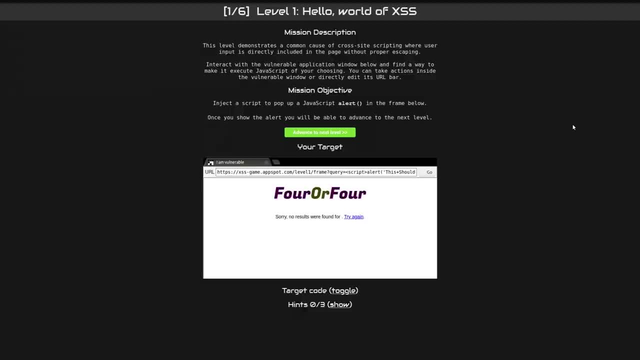 Now you're probably thinking that this isn't a very big deal And, in this particular case, just a website that isn't actually connected to anything. There's really nothing important that I can try to pull out of this right. So that example is called a reflective CSS attack. 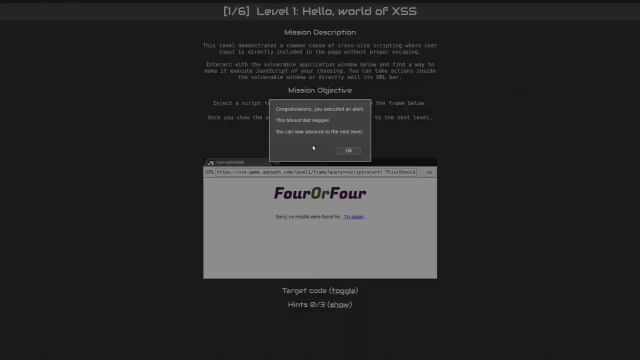 because we're just you know, it's being reflected right here back at us. But this can still be used for some nasty stuff like stealing cookies. But there's another type of cross site scripting attack, called a stored cross site scripting attack. So this is where, instead of the results of the injection just being sent right back to us, 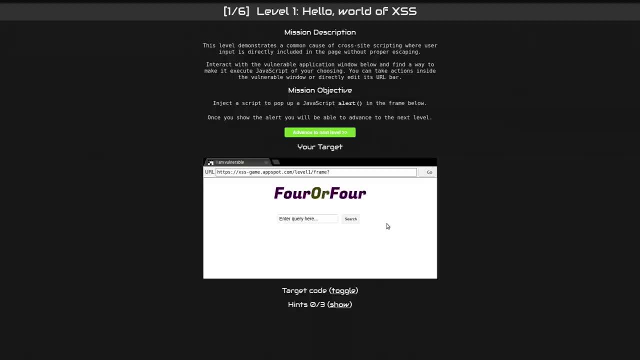 immediately. the input actually gets stored on the website and some kind of a database And it isn't executed until some other end user, or even you, visits that part of a web page or clicks a button that's going to pull some information out of that database. 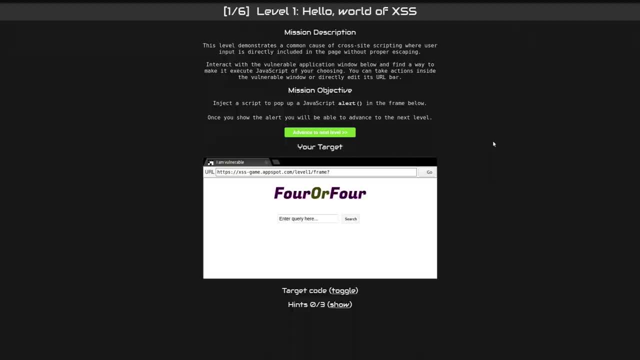 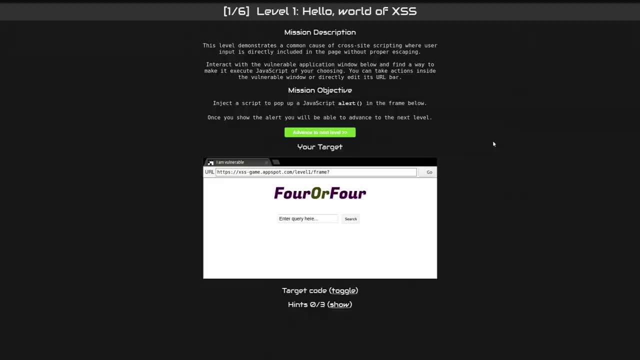 can just go back and do that, And then they can just go back and do that, And then they can just go back and do that somewhere on a website that they know a person is going to go to later. maybe it's going to be like the new product section of Amazon or some other website. 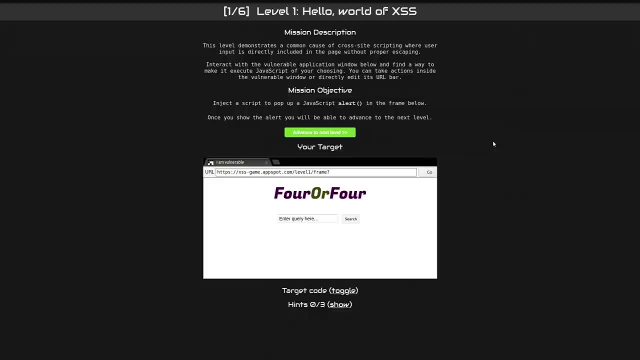 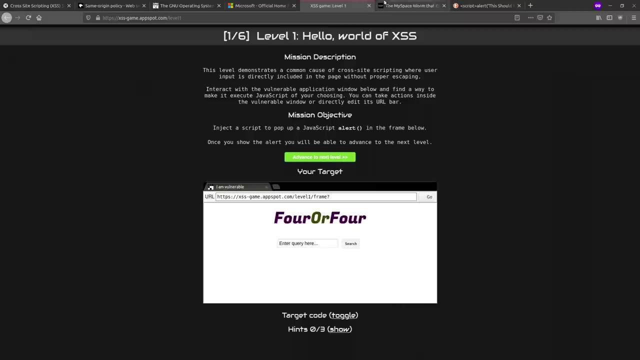 or they might have it resting in the web page to be executed later, Like maybe they'll put it under winter jackets when it's the middle of the summertime and then later on they're going to go and execute that once they visit the page. So the most famous example of something like this is: 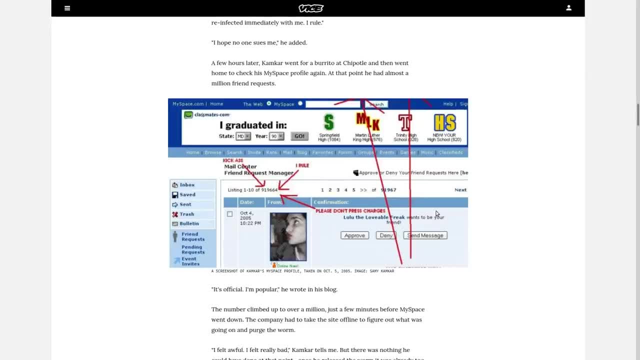 probably the Sammy worm. So this was a cross-site scripting worm that took advantage of a vulnerability that MySpace had back in 2005.. Now, luckily, this worm was relatively harmless, like it didn't really do anything too too bad. Basically, it just updated your bio on MySpace to include 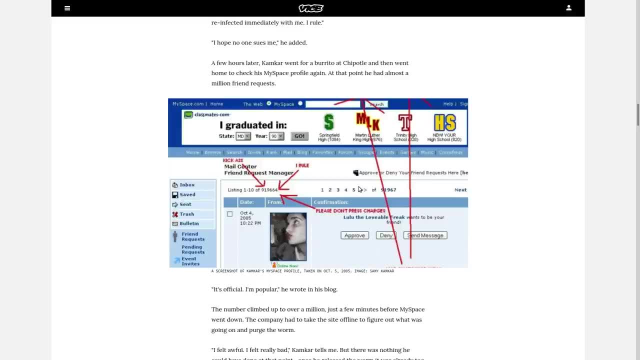 at the bottom of it the words Sammy is my hero, and then it would be at the end of your bio and it would send a friend request to Sammy. So you know this spread really, really fast, because after it modified your bio, the script would then embed itself into your profile page. 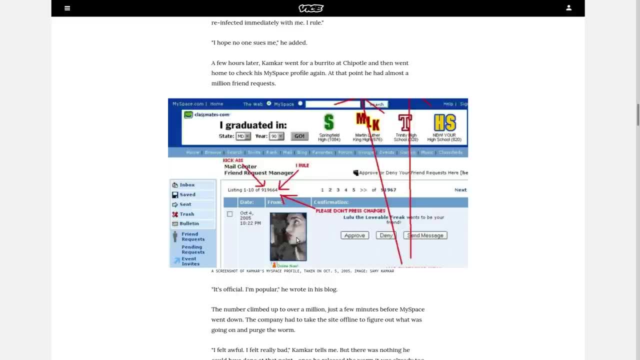 So there would be some kind of patient zero who first saw this on Sammy's page, Like I think he put it into his bio first, and now anybody who's going to that person's page, it executes. and then, if you went to that person's page, anyone who's looking at your page now, it's going to execute. 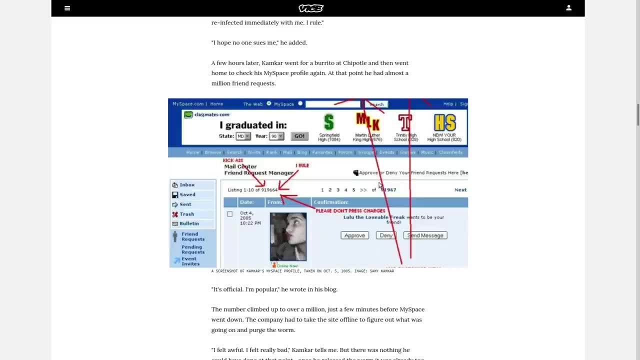 and so on and so forth. That's the reason why I think it was like one hour like. this screenshot is from an hour or so after he launched the worm. You can see how many friend requests he has now: so 919,000.. And again, this was back in the early days of the internet, before a whole lot of people were. 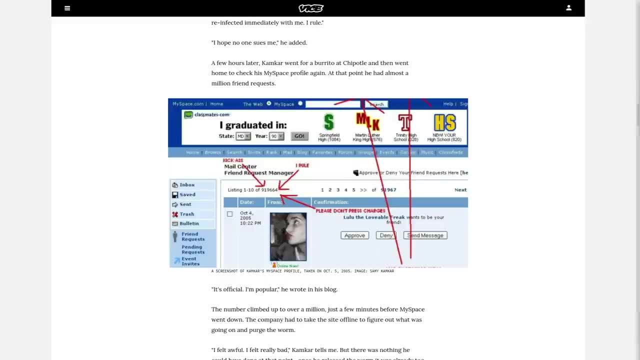 on it. So, yeah, it spread really, really quickly and since this is JavaScript, it could do anything in the web page. It could have been stealing login credentials, It could have been redirecting people to other websites. There's really no limit- And there's also a DOM based cross-site. 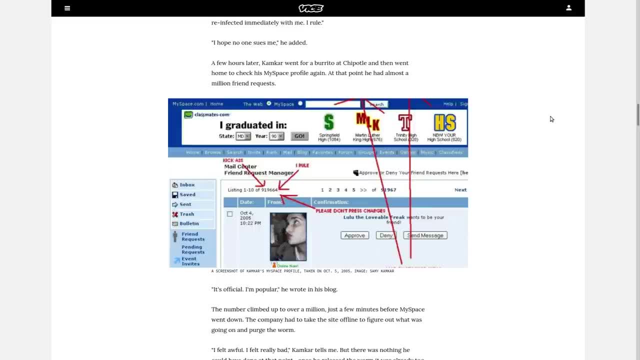 scripting attack which happens entirely in the client side and it doesn't necessarily reflect anything back to the victim when they execute it. But that could be done by just sending a sort of a request to the client and then it would send it back to the client. 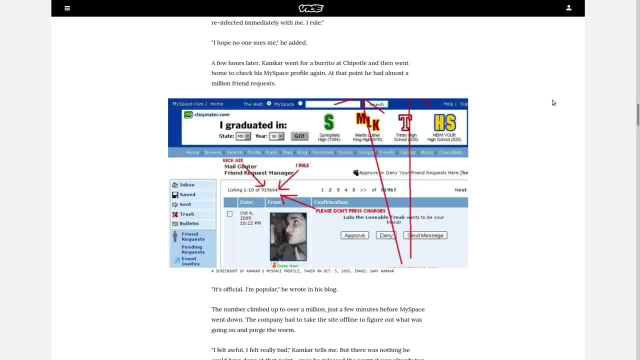 It's sort of like malicious link to the victim so that the client side code runs in an unexpected manner. The page itself doesn't change, so it's not reflected, but the client side code contained in the page is going to execute differently And there's mutation. cross-site scripting, where the 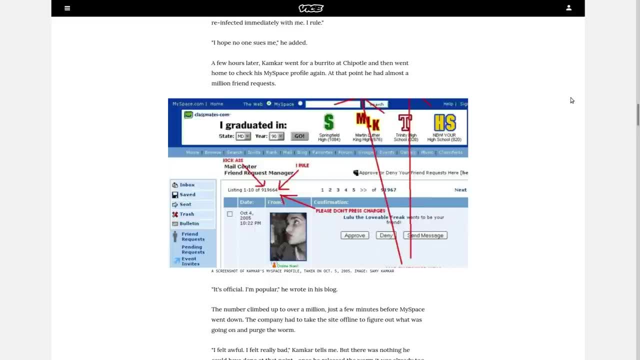 user input is changed by the browser before inserting it into the DOM, which can sometimes lead to cross-site scripting if it's implemented incorrectly. So yeah, Cross-site scripting. It's a very serious problem and you need to take a lot of time when developing. 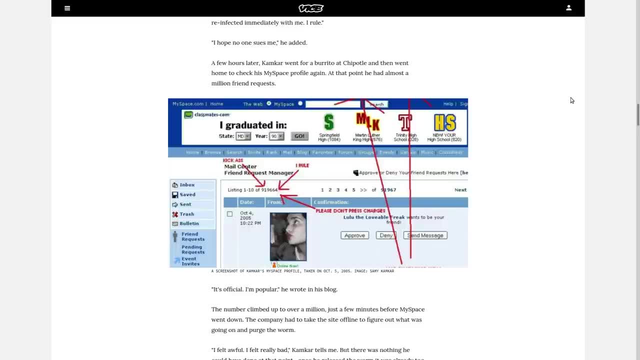 your web app to make sure that it isn't vulnerable to this. That's actually one of the common things that you should be doing whenever you're designing web apps in general is, you know you take maybe 30 percent or so of the time to actually develop it, but then the rest of the time you're spending 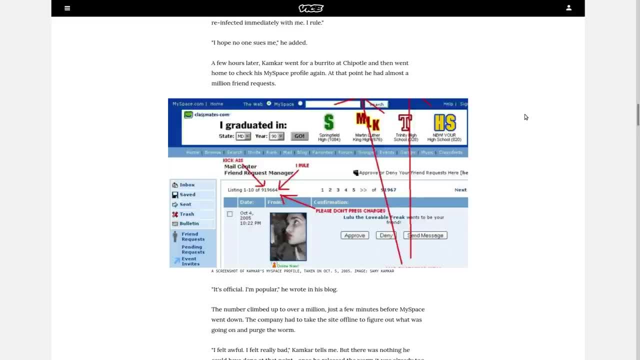 securing it, maybe pen testing it yourself to make sure that there aren't any vulnerabilities in it, or you could hire people to pen test it. It's obviously going to be much better and much cheaper for you to figure that type of stuff out before having to like pay lawsuits and stuff to your